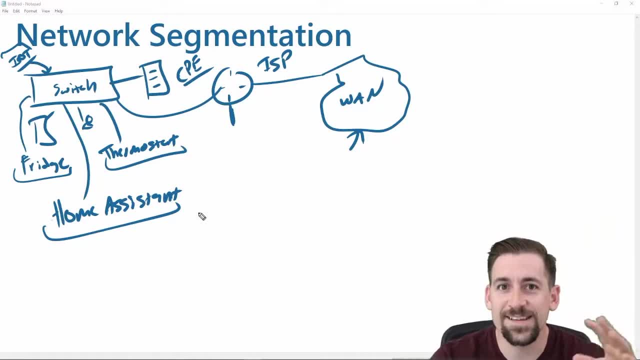 firmware right. Oftentimes, if we're not cognizant of the types of devices we're buying and putting on our network- and this happens in both the home office environment and in the enterprise environment- if we're not cognizant of this fact, then we may pick up devices that have known issues or companies that don't push out firmware updates when vulnerabilities are discovered, and these types of things very, very common. Also, vulnerabilities are discovered sometimes in firmware or packages that were utilized by a number of companies and are pervasive and aren't fixed very much at all, And this happens more often in IoT device. 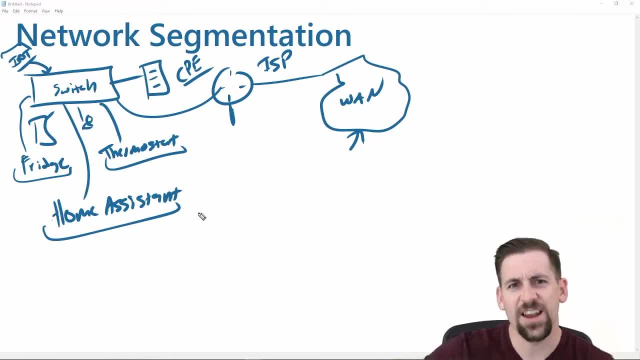 infrastructures than it does in other infrastructures. This is why I'm focusing specifically on IoT for network segmentation today. right, Okay, so I've established why I would put these on the network. I've established why I don't want them to be on the same network as my main work PC and a server. 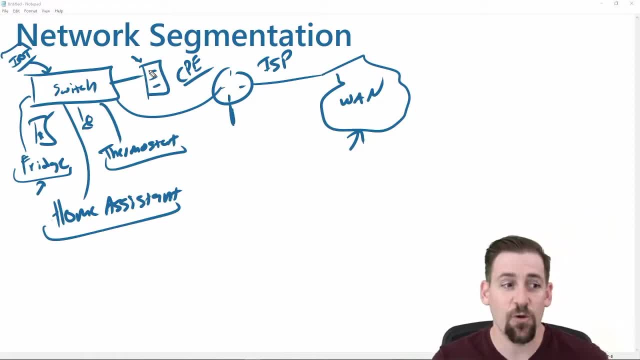 or a printer or some other device that's being utilized for work purposes, for example, right- And so I need a primary LAN and I need, let's say just in this case, right- a segmented network for IoT devices that is separated from the primary LAN for security. 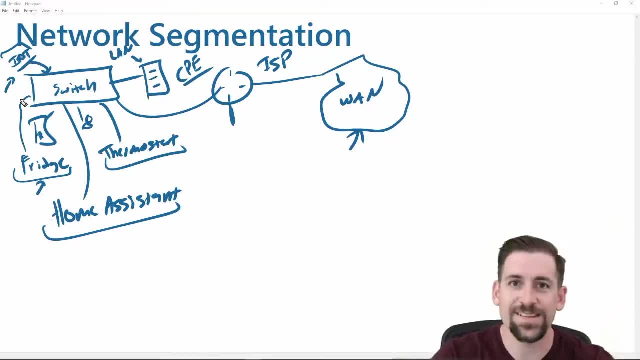 purposes specifically, We could separate it for a number of other reasons and do quality assurance and policy of the traffic and all these other things, But let's say we're talking specifically about network security and segmentation here. Okay, so there's one way I could do this is I could. 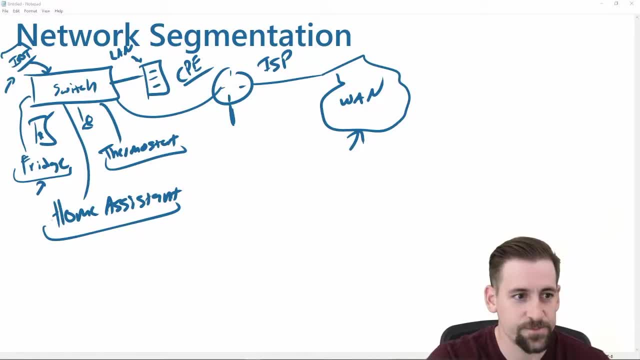 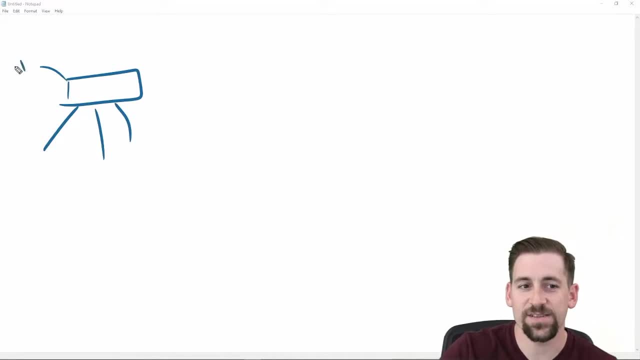 have two physically separate networks, right, So I could take and plug all of these devices into a switch or a wireless access point: IoT devices, home assistant, camera, thermostat. I could plug this switch into a router and I could take another interface on that router. 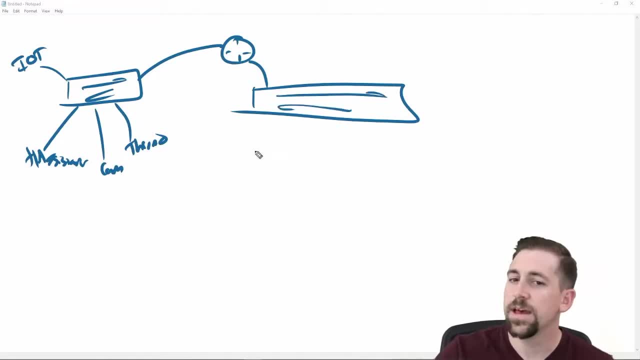 connected to a switch and then hook up my PC via Cat5 or high throughput fiber. whatever I want to do depends upon the data transfer rates I need and some other server over here, And then I could have my WAN connection. In this case, I have a single router acting in my segmentation and security. 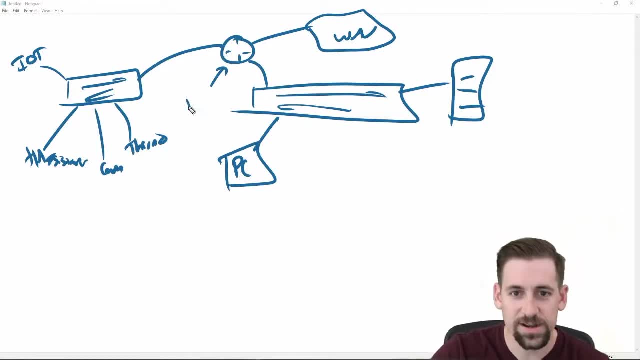 from my segmentation and security perspective as a router, firewall, Hybrid, And these IoT devices can now communicate to the WAN. If I were to be, you know, if I were out on the WAN? let's say Travis IQ is out here on the WAN and needs to. 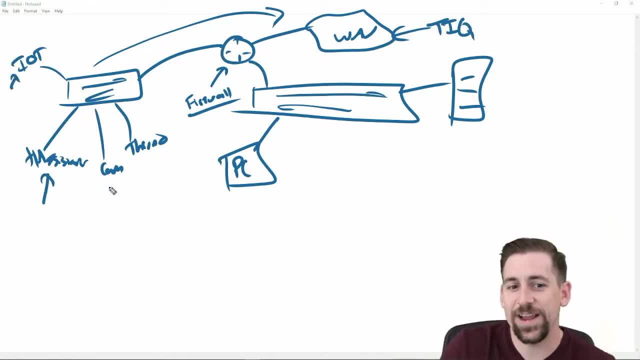 talk to his home automation server that is aggregating information from all these other IoT devices And I forward. I punch a hole in my firewall and forward traffic from port 443 to 8123, which is the default port for home assistant, And I log in and I get all this information. 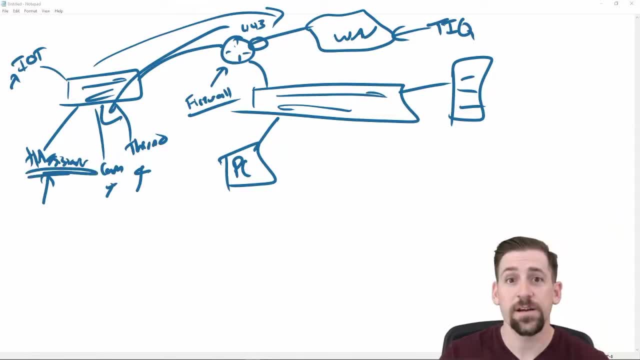 Now this server is actually exposed right. This port is now being forwarded to this service here And anyone who attempts to connect to my network via that port is going to be forwarded to this service. This is why we set up strong usernames and passwords and multi-factor authentication. 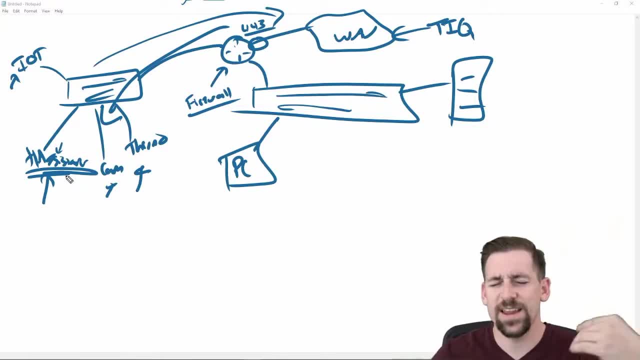 So that, although we understand that this device is exposed, it is a potential security risk, more so than these other devices here. It is secured and segmented, So we have layers of security and we'll talk about things like defense in depth on this channel at some point as well. 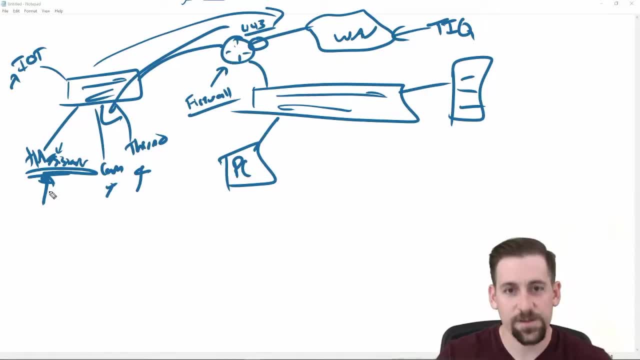 Okay, So this is one mechanism of segmenting the network. If I needed this server, or if I needed this PC to be able to talk to this server, if I were to in the case of home assistant, I needed to update a configuration and the way that I would update. 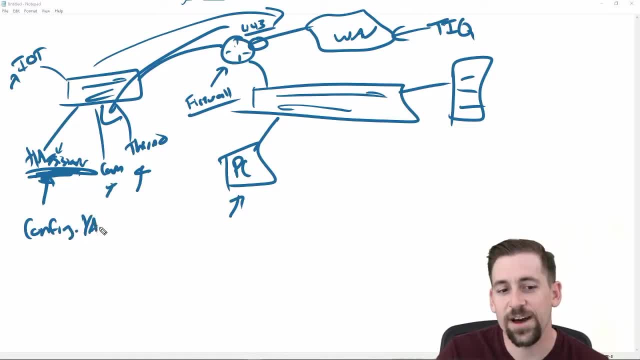 configurations in home assistant, The configyaml file, And so I needed to do some configyaml updates And I wanted to use something like windows SMB to update the configyaml file- basically windows server message block- So I could connect directly to it like it were a folder on my PC here directly. I could do. 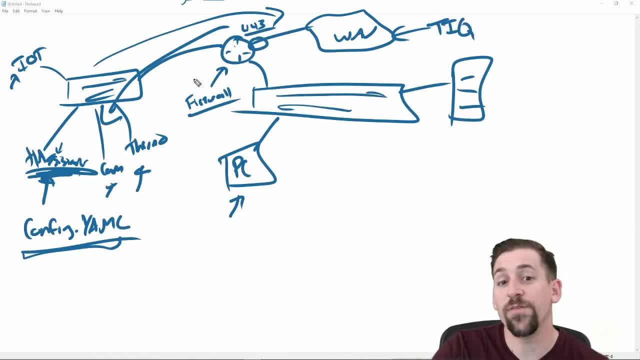 that I would have to do one of a few things I could do: white listing of those IPs and directions. We'll talk about firewall configuration another time. I could white list an IP and a port number, or I could do established connections- a number of different things. 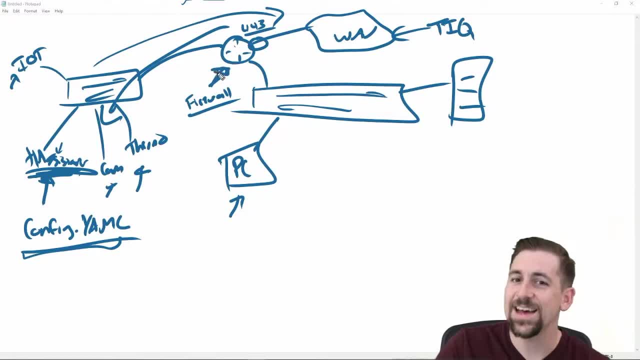 But I would have to allow explicitly that connection from this device to this device within that firewall config. You'd say: how would you do that, Travis? Well, it would vary from NOS to NOS network operating system or firewall operating system to firewall. 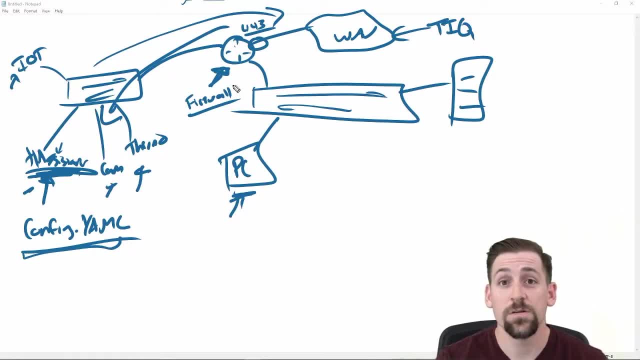 Juniper, Palo Alto, Fortinet, Cisco, PFSense, Untangle, pick your device. Okay, I said I could do this one of two ways, So what's the second way, Travis? Well, I don't have a ton of ports sitting off my small router in a smaller or medium business. 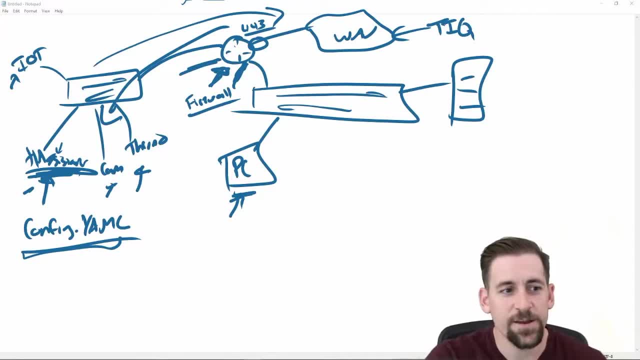 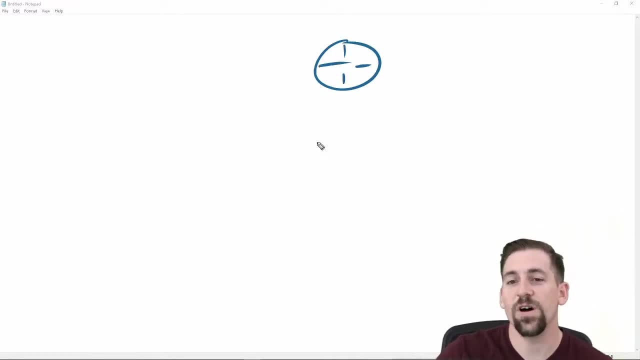 infrastructure to segment the network like this. Usually, especially in a small office environment, I'm going to have one router or maybe one and one set up in high availability and redundancy. But let's say, I'm going to have one router and one, setup in high availability and redundancy, But 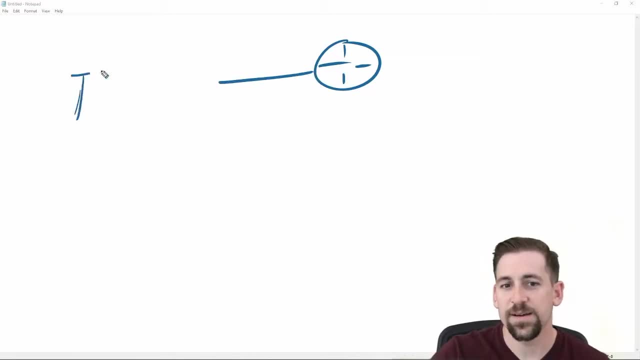 let's say I'm going to have one router and one setup in high availability and redundancy. But let's say one router connected to a big backbone switch in my office And I've got a bunch of devices connected to this that want to get out to the land. 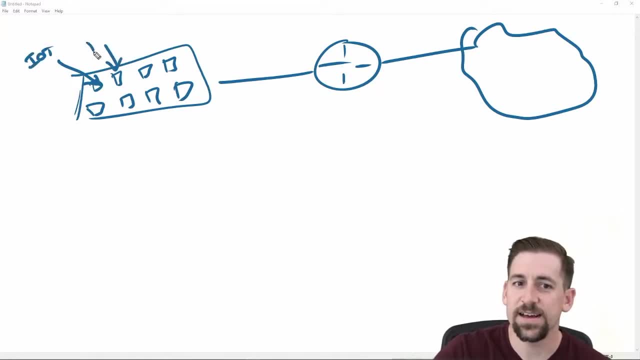 And I've got these IoT devices- IoT, IoT, IoT- These are going to be on my IoT segment. And then I've got these other devices here- PC server, backup server- that are going to be on another segment here. 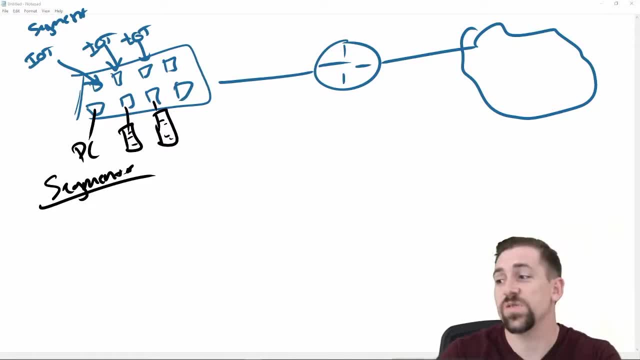 I can instead do what is known as virtual segmentation. Virtual means- we use the term logical, Logical means in software. So in software we define this segmentation. Sorry, I should probably do this in the right color. In software we define this segmentation. 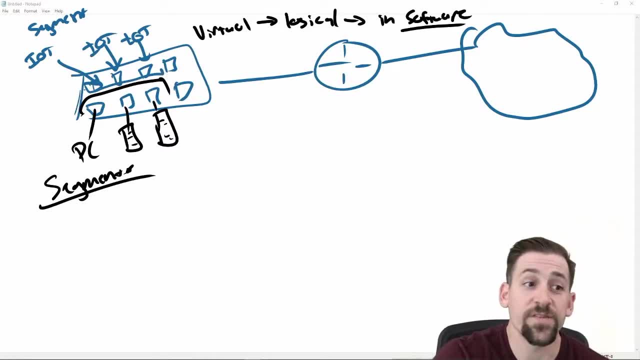 like this, And there's a term for this. These would be different local area networks at that point, So they would be virtual local area networks, or VLANs, And so what I can do is I can configure multiple VLANs on this switch. Switches can segment the network using VLANs. 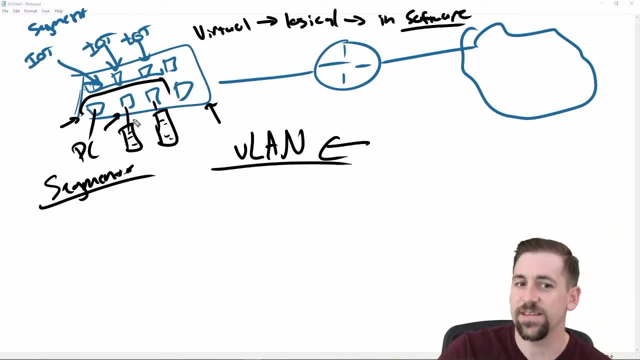 And I can associate this PC, this server and this server with VLAN 5.. And I can associate my IoT VLAN with VLAN 999,, let's say, And what this means is? they are Essentially, this is essentially the same as segmenting them with a router, where they have 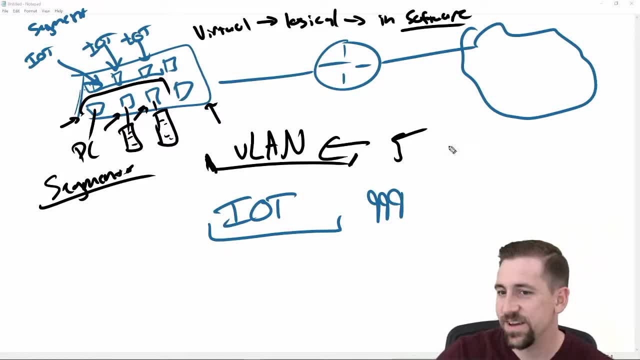 their own networks. So that means that they would have their own IP address ranges. So this could be the 192.168.1.0 address range And this could be the 192.168.2.0.. So one thing that we know about. 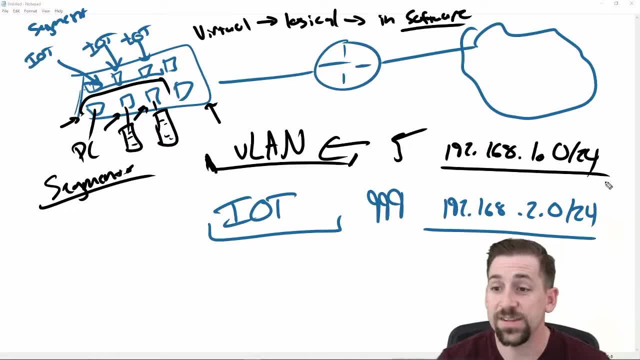 separate address ranges like this right The 192.168.1 and the 192.168.2 is, they require a router to communicate with the two, And so in this scenario here, where I just have a switch, let's say I'm not connected to this. 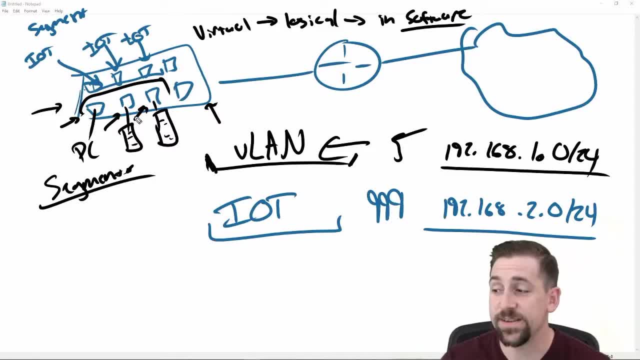 router. right, Those two networks actually can't communicate, right, Because they're separated in software in the device and across those boundaries, right, We would need a router to route that traffic, And so what we can do is have R1 here, route the traffic for us, And 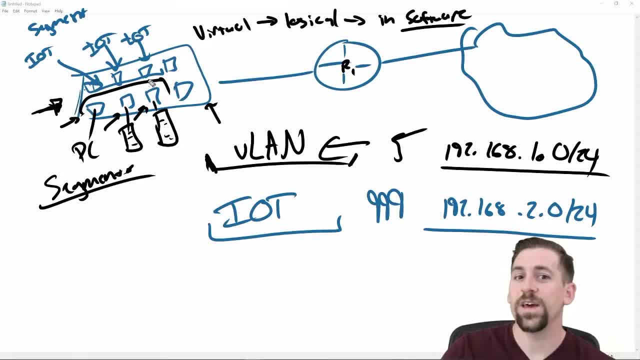 then we have network segmentation, with a device that's not necessarily innately intended to segment the network, And we have a device facilitating communication between those networks, if we so desire. If you're going to set it up like this, what you're likely going to have, 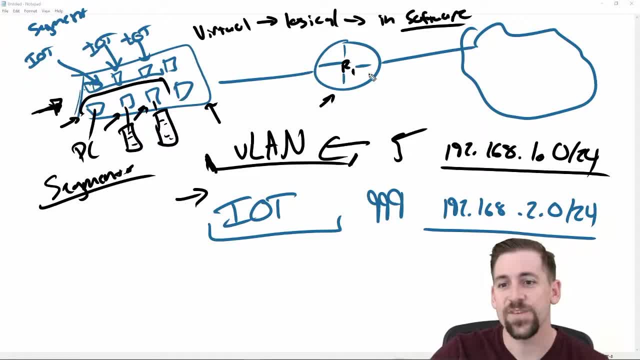 in this case, barring some specialized cases, is this router is going to prevent communication between these two networks until you explicitly allow it. right, And that would be part of our functionality, And so we would have firewall rules preventing the connection between these two networks. You would say, well, maybe in some core routers and some core implementations. 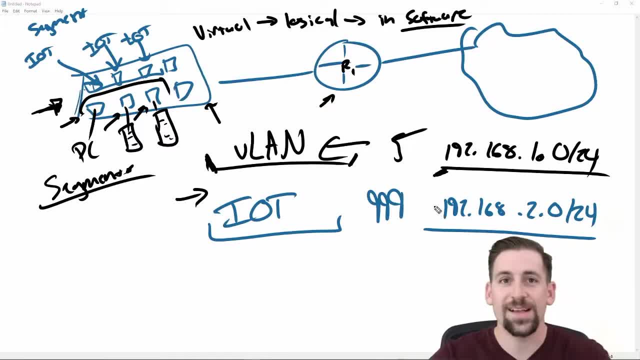 that might not necessarily be the case, And I agree with you, But in our small, medium enterprise example here, that would definitely be the case. And so now you've got your IoT devices, you've got an IoT automation and home automation utility. 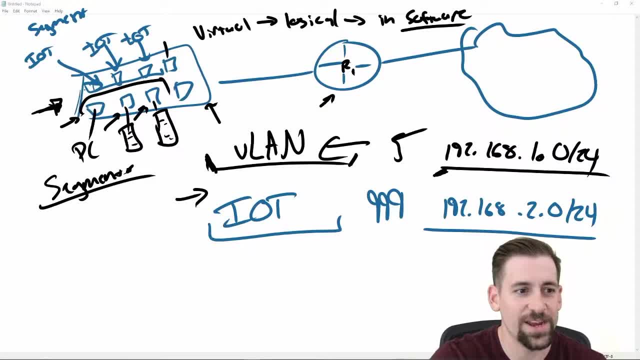 Hold on, sorry, wrong color. You've got a home automation utility here That sits here too, And I want to manage it with my PC. I still have to punch a hole in this firewall to allow these two devices to communicate. We'll talk about how we would facilitate this and how you. 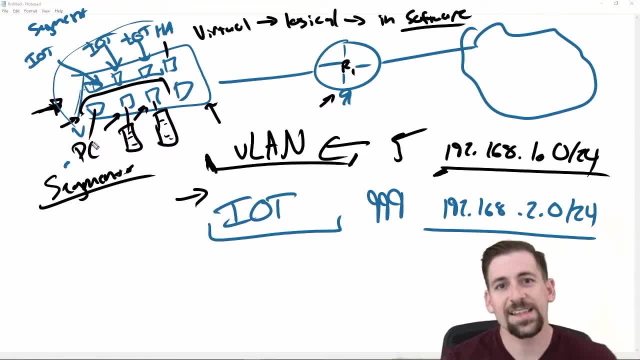 facilitate intervailing routing with a single router or router on a stick like this, with things like sub interfaces and stuff like that at a later date, But as of now, this is sufficient for our discussion of network segmentation. If you'd like to see more discussion of cybersecurity topics, networking topics,